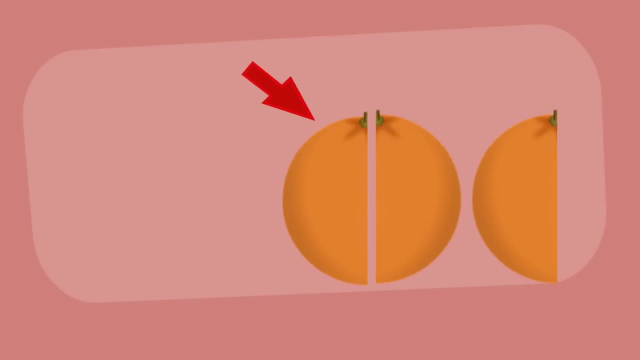 an orange: One half, two halves, three halves. You can see that three halves is larger than one whole, because we have one whole orange and an extra half. Three halves is an improper fraction. Improper fractions have a numerator larger than their denominator. An improper. 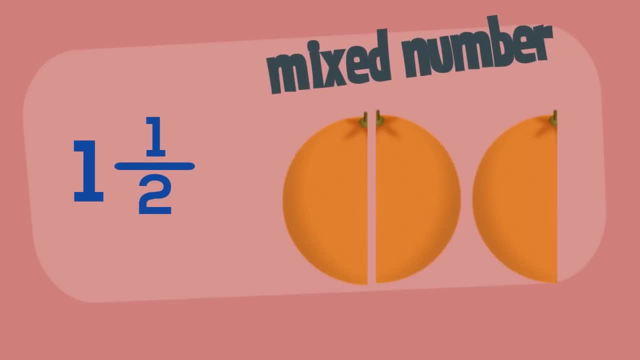 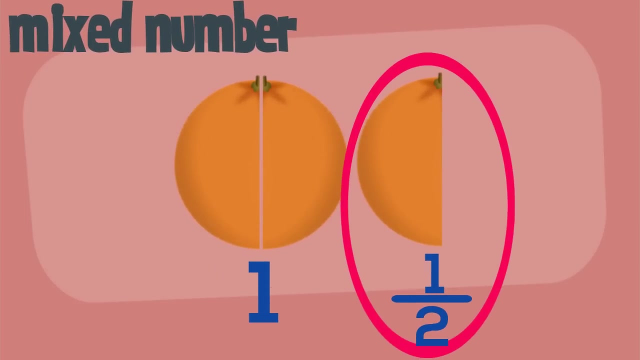 fraction can also be expressed as an improper fraction. What is a mixed number? It's called a mixed number because it's a mix of a whole number and a fraction. How many wholes do we have One? How many extra halves do we have One? 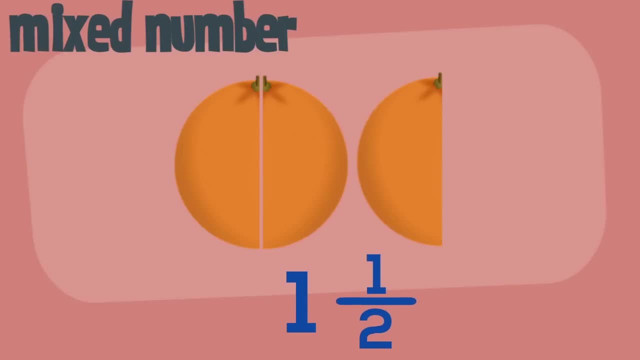 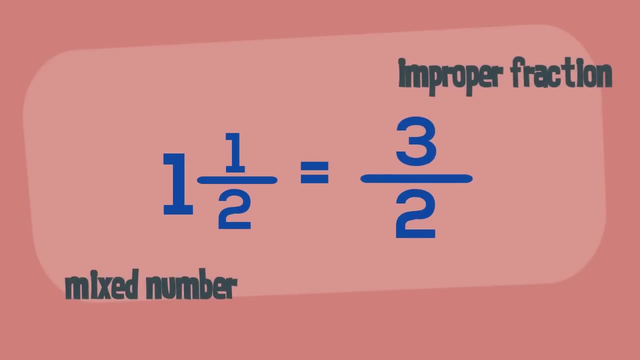 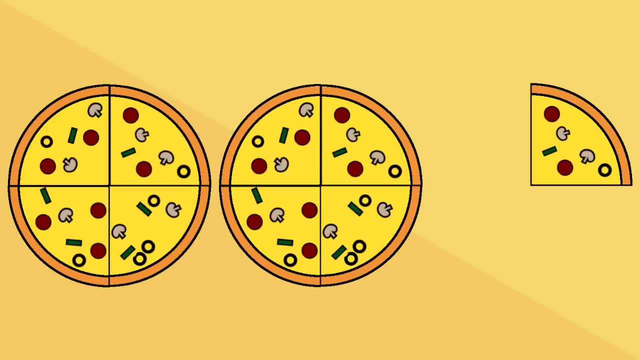 One whole and one half. The mixed number is one and a half. One and a half is the same as three halves. Let's take a look at another example. What fraction have these pizzas been cut into? That's right quarters. Let's count how many quarters we have: One quarter, two quarters. 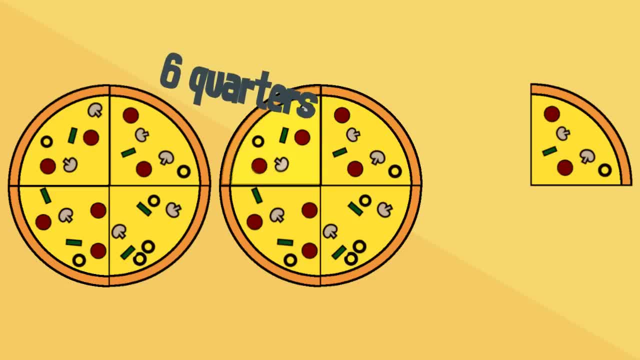 three quarters, four quarters, five quarters, six quarters, seven quarters, eight quarters, nine quarters. We have nine quarters. This is an improper fraction, because the numerator is larger than the denominator. Let's think about how we could write this as a mixed number. How many wholes are there? 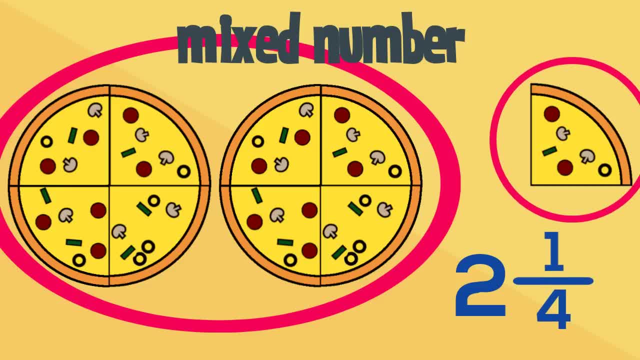 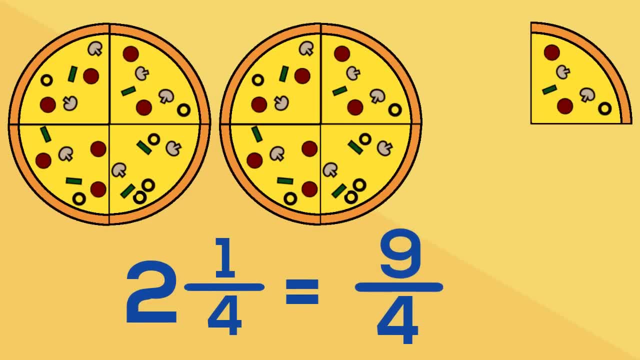 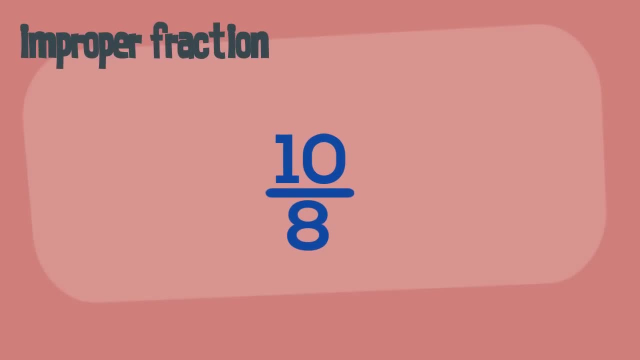 Two. How many extra quarters are there left? One: The mixed number is two and one quarter. Two and one quarter is the same as nine quarters. Here's another improper fraction. Let's convert this improper fraction to a mixed number. We are working with eighths. 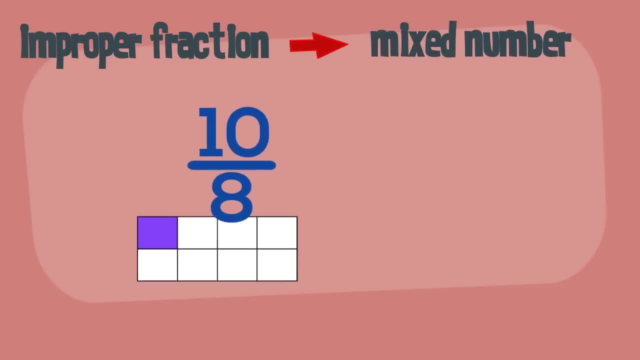 Our fraction has ten of them: One eighth, Two eighths, Three eighths, Four eighths, Five eighths, Six eighths, Seven eighths, Eight, eighths, Eight eighths is one whole. Nine eighths, Ten eighths: There is one whole. 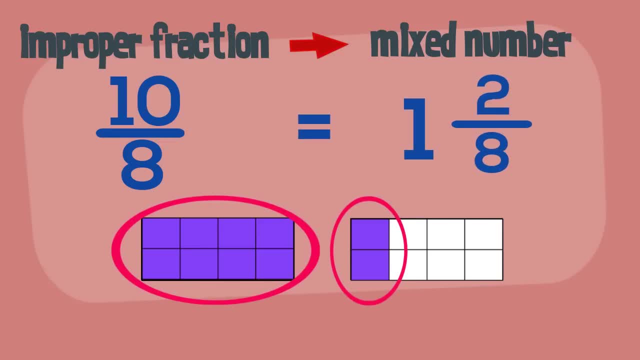 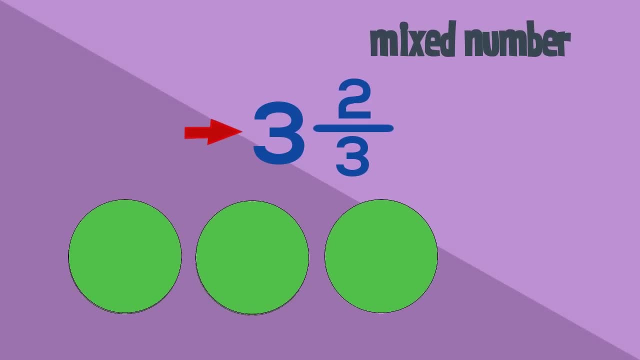 and two eighths. The mixed number is one and two eighths. Here we have a mixed number. It's telling us that we have three whole and two thirdss. How can we express this? this as an improper fraction? Easy: We count how many thirds we have all together. We know. 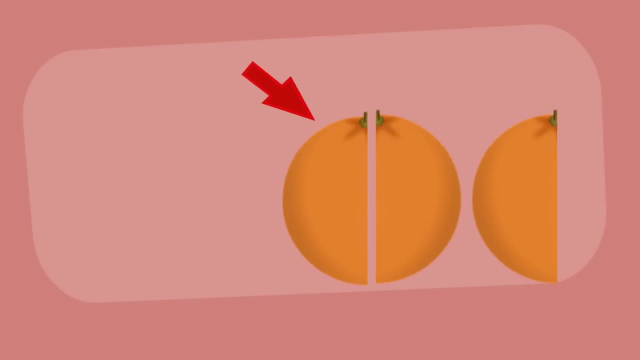 an orange: One half, two halves, three halves. You can see that three halves is larger than one whole, because we have one whole orange and an extra half. Three halves is an improper fraction. Improper fractions have a numerator larger than their denominator. An improper. 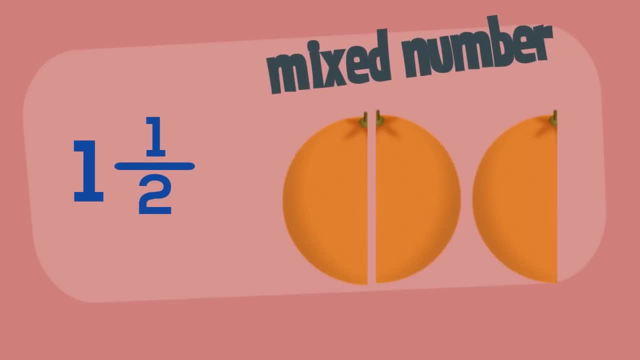 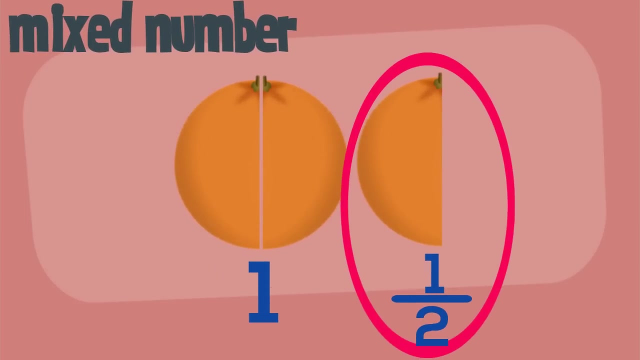 fraction can also be expressed as an improper fraction. What is a mixed number? It's called a mixed number because it's a mix of a whole number and a fraction. How many wholes do we have One? How many extra halves do we have One? 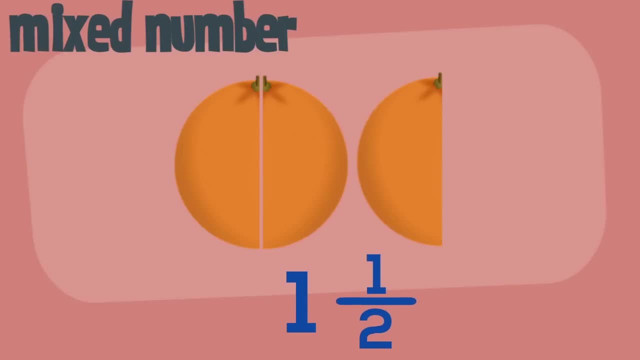 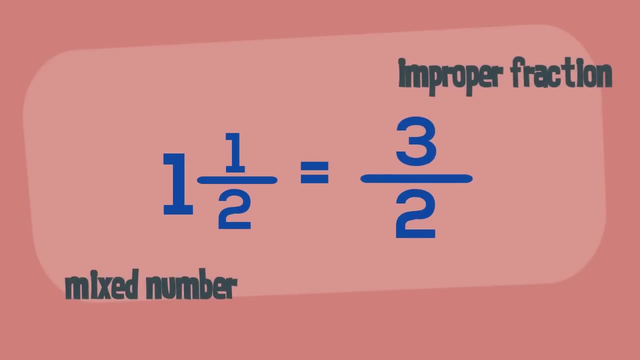 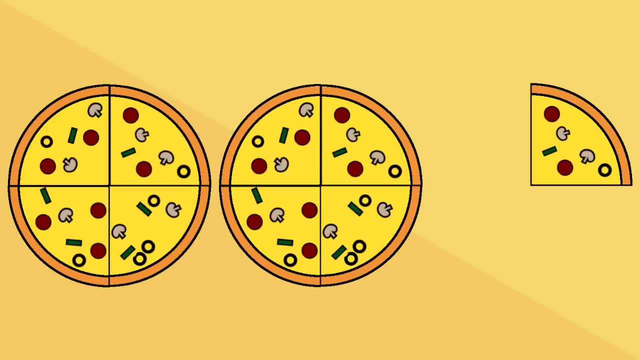 One whole and one half. The mixed number is one and a half. One and a half is the same as three halves. Let's take a look at another example. What fraction have these pizzas been cut into? That's right quarters. Let's count how many quarters we have: One quarter, two quarters. 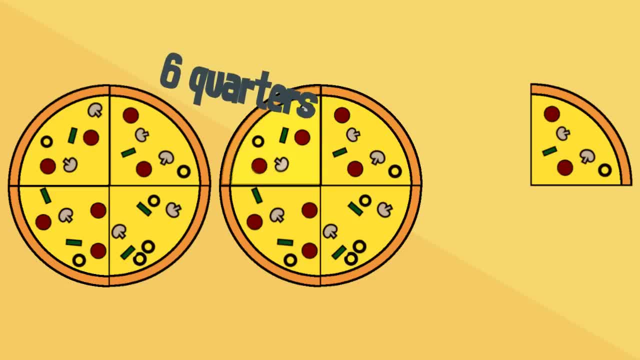 three quarters, four quarters, five quarters, six quarters, seven quarters, eight quarters, nine quarters. We have nine quarters. This is an improper fraction, because the numerator is larger than the denominator. Let's think about how we could write this as a mixed number. How many wholes are there? 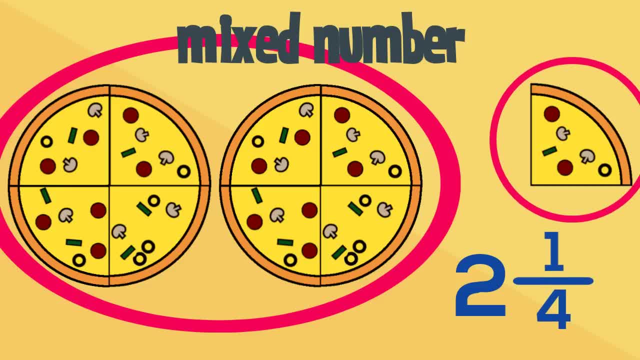 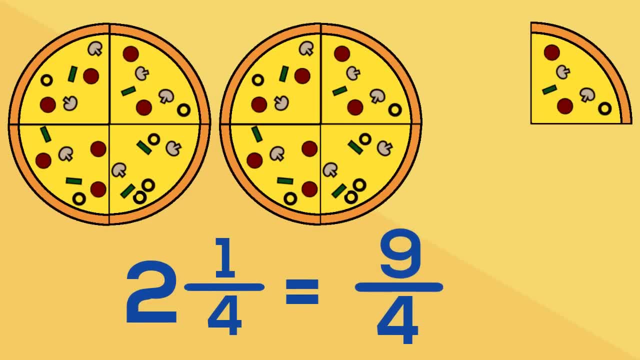 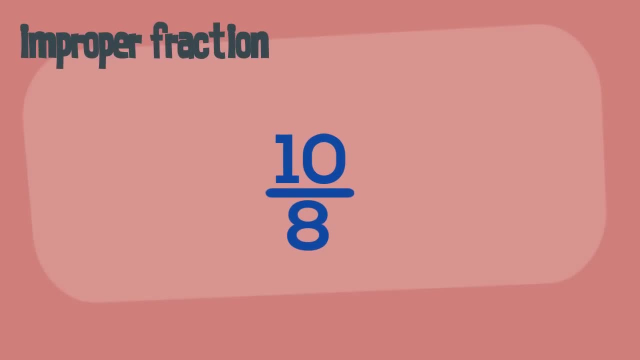 Two. How many extra quarters are there left? One: The mixed number is two and one quarter. Two and one quarter is the same as nine quarters. Here's another improper fraction. Let's convert this improper fraction to a mixed number. We are working with eighths. 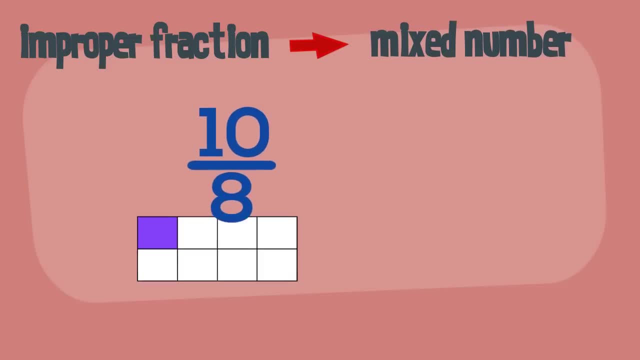 Our fraction has ten of them: One eighth, two eighths, three eighths, four eighths, five, eighths, six, eighths, seven, eighths, eight, eighths, Eight, eighths is one whole. 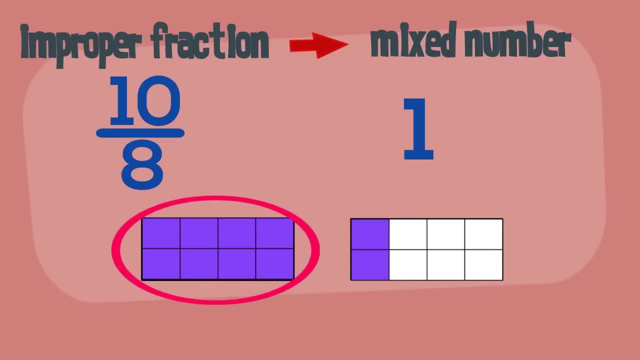 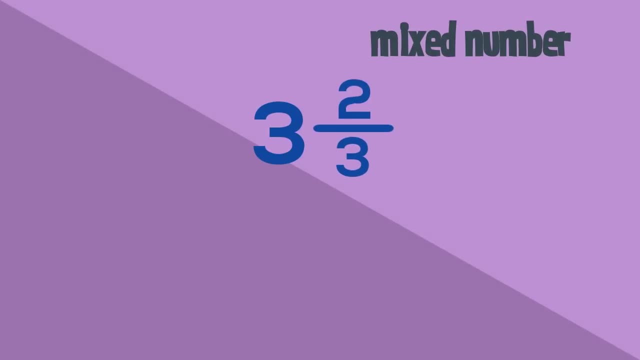 Nine eighths, 10 eighths. There is one whole and two eighths. The mixed number is one and two eighths. Here we have a mixed number. It's telling us that we have three whole and two thirds.